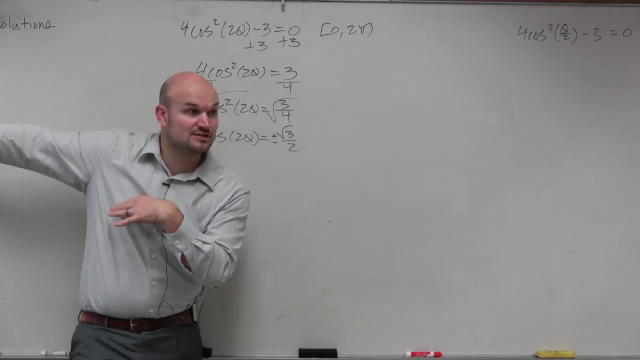 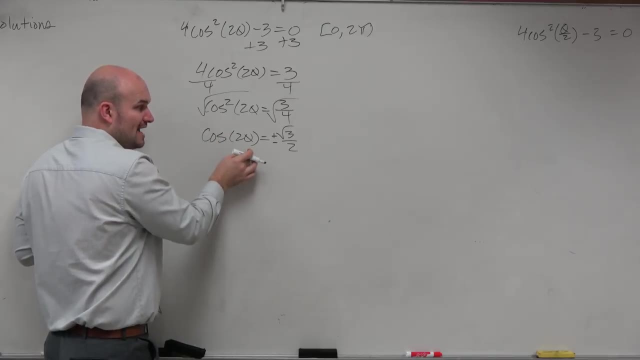 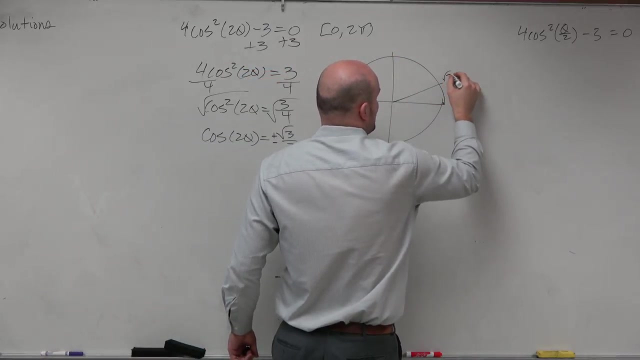 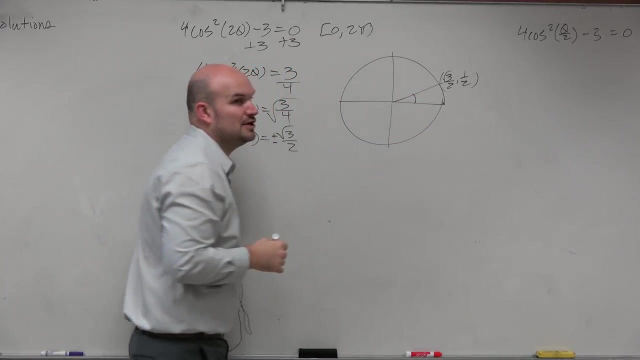 Right Now. let's go back to all. let's go back to finding the solutions. When does cosine of what angle? forget about the 2 again, Just forget about the 2. Cosine of what angle gives you square root of 3 over 2? So again we go back to our unit circle and we say: when is cosine equal to square root of 3 over 2?? It's this angle. I just got to remember what that angle is by the unit circle And the angle is Pi over 6. And I know that it's plus or minus. So every other angle that has that same reference angle is the same reference angle. 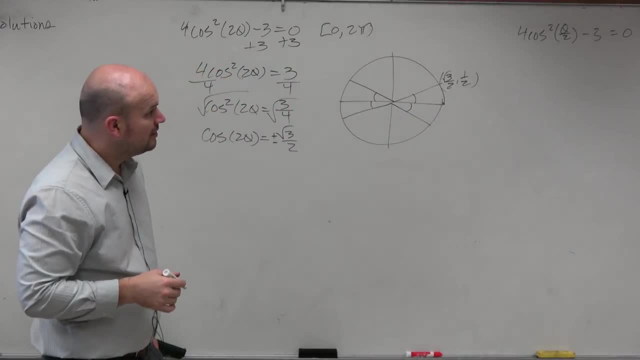 Is. cosine is either going to equal plus or minus square root of 3 over 2? So therefore I have to figure out all these angles Again. if you're confused on this, just let me know. But I know yes. 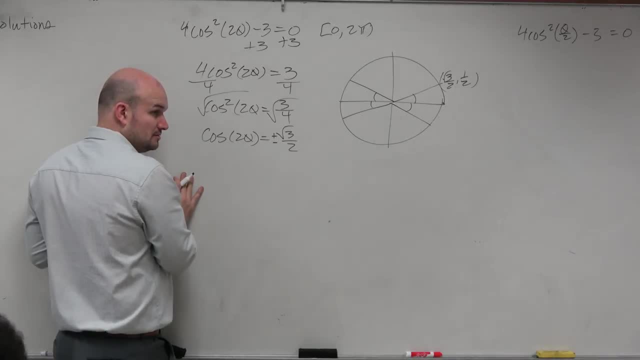 Generally, could you square root before you divided? Huh, Generally, could you square root before you divided? No, Dividing Like you could square root before cosine over 2. 4x squared equals 3.. You don't take the square root for there. 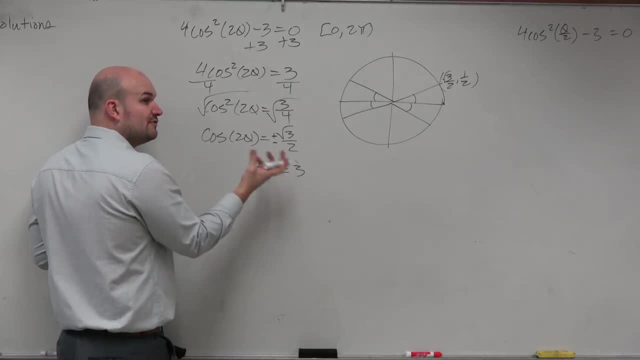 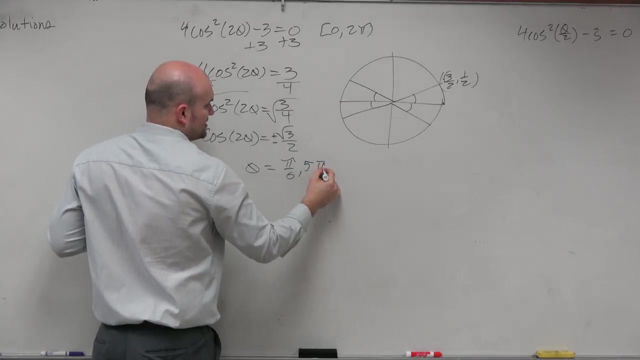 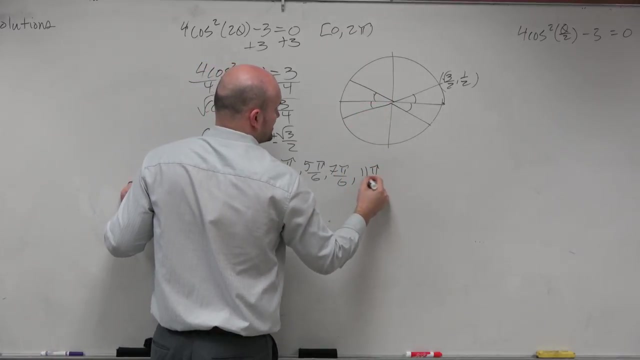 I mean, it works, We want to. just, you always want to Use the reverse order of operations. Okay, All right. So basically here we have: theta equals. our answers from our last example are: pi over 6,, which is this answer. 5 pi over 6,, which is that answer. 7 pi over 6,, which is this answer. and 11 pi over 6,, which is that answer. 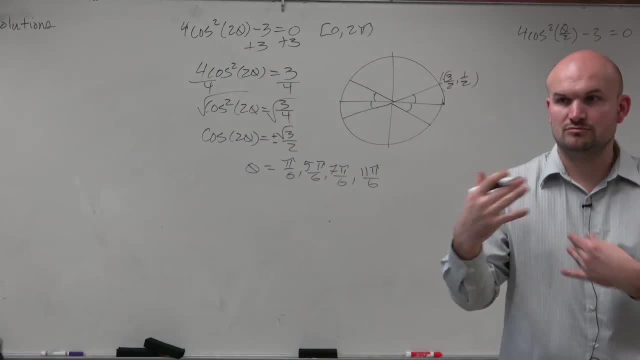 Is everybody good with this? Again, I haven't taught anything. I'm just regurgitating what we've already done. Yes, Now, the difference here is: now we're going to change the type, now we're going to change a little bit. 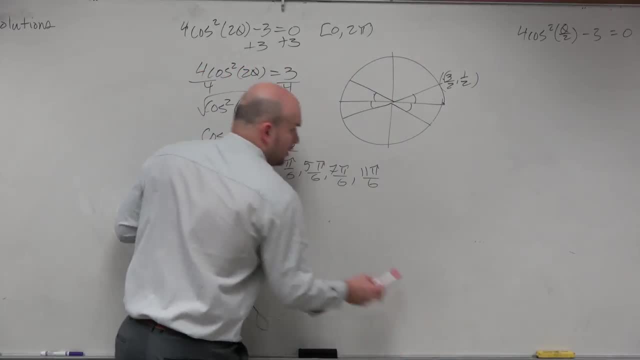 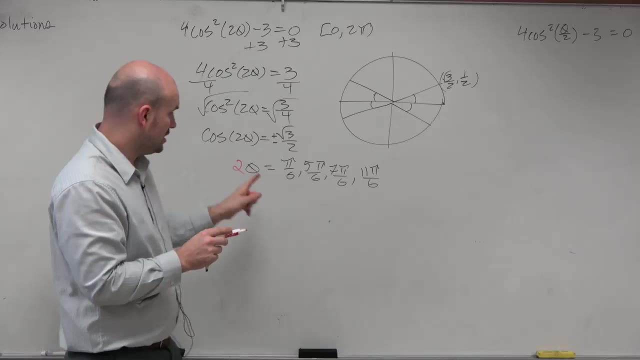 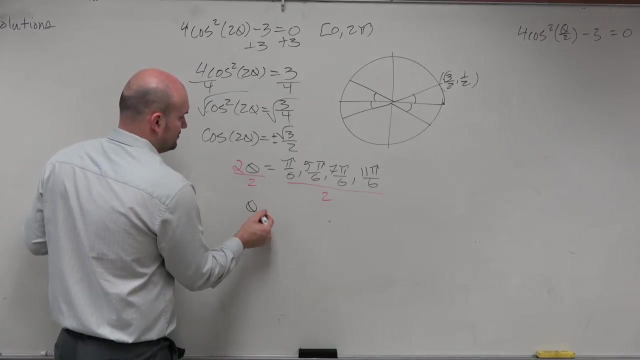 Because the problem isn't saying solve for theta. The problem is now saying solve for 2 theta. So all we have to do extra is just undo multiplying by 2.. So if we divide by 2, theta equals pi over 12,, 5 pi over 6.. 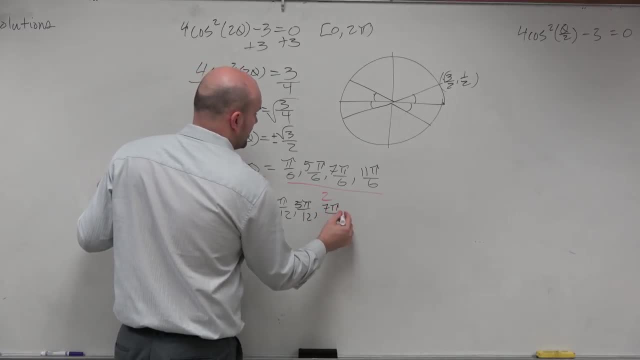 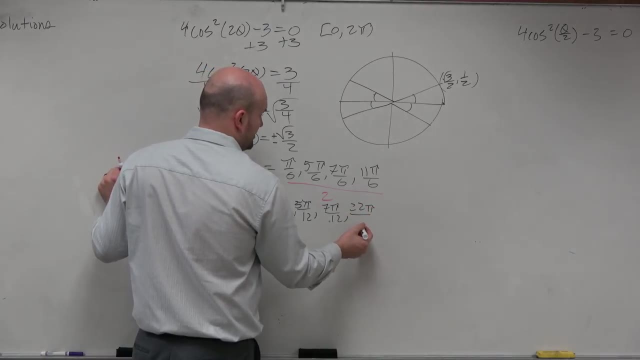 7 pi over 12,, 7 pi over 12, and 22 pi over 12.. And many students would say, okay, I'm good, That's actually easy, I understand it. But the problem is that's not all the answers. 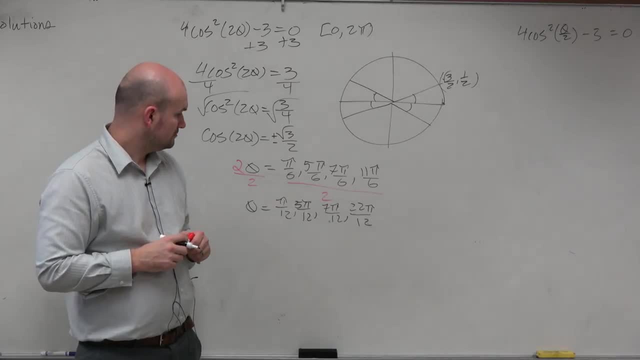 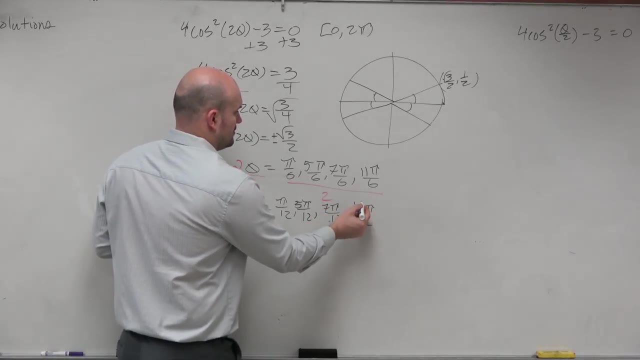 Yes, Question. Okay, so you went from 11 to 22,, but you didn't go 5 to 10. Or 5 to Sorry, that's supposed to be 11.. Yeah, Okay, And I thought you were going to divide it out. 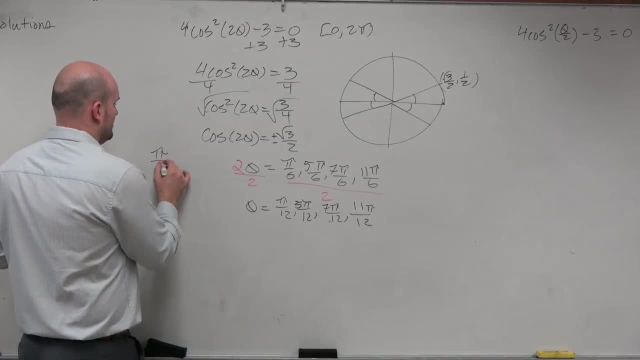 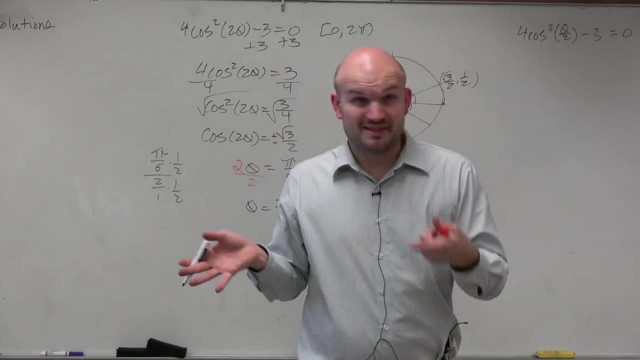 So just remember: pi over 6 divided by 2 is the same thing as 2 over 1, multiplied by the reciprocal. Okay, Now, that's not all the answers though, But that's at least the easiest four answers to find. 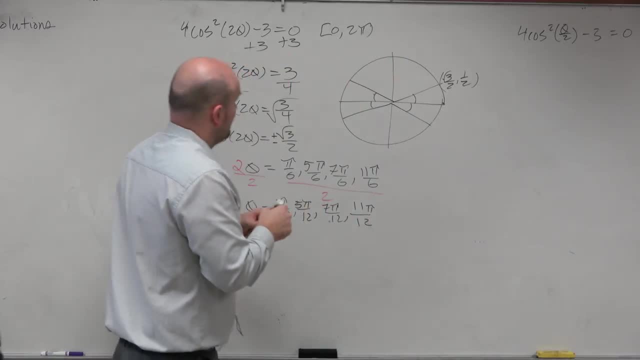 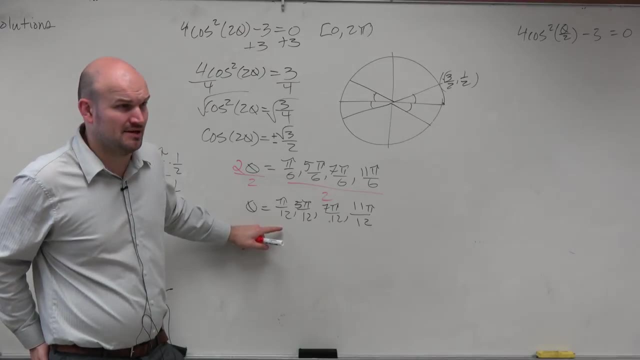 So we've got to find all the other answers Because, think about it, guys, If I said I want to find all the answers between 0 and 2 pi, we're now dealing with a denominator of 12.. We haven't dealt with many problems with a denominator of 12.. Would you guys agree? 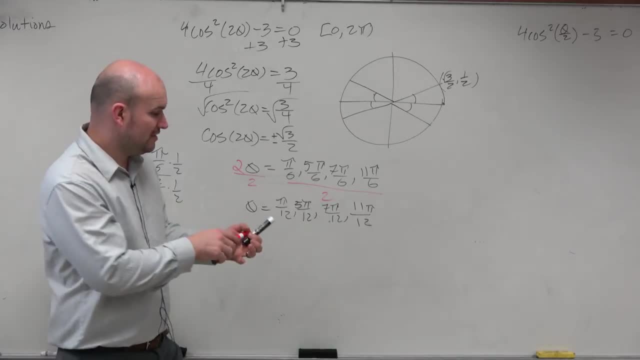 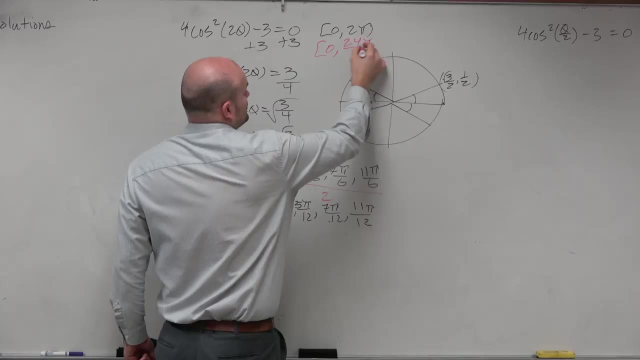 Right. So this is kind of a little new uncharted territory for us. However, I would say I would say we're pretty comfortable with understanding that 0 to 2 pi then is 24 pi over 12.. 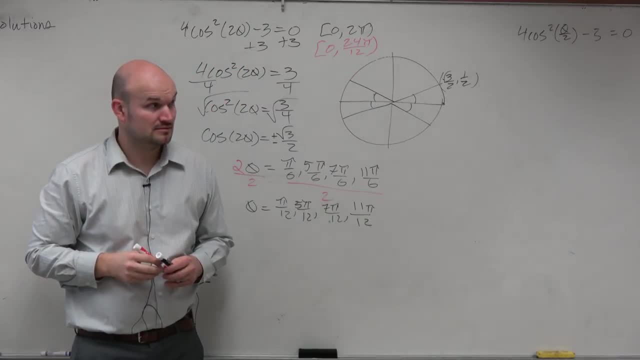 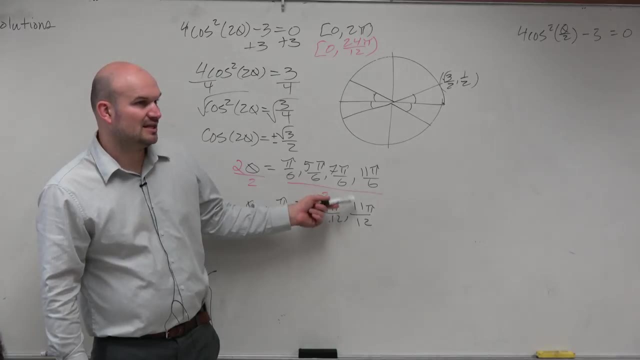 Would you guys agree with me at least on that statement? Yeah, Does that make sense? 24 divided by 12 is 2?. Look at our answers. The highest answer we got is 11 pi over 12.. Do you think there may be some? 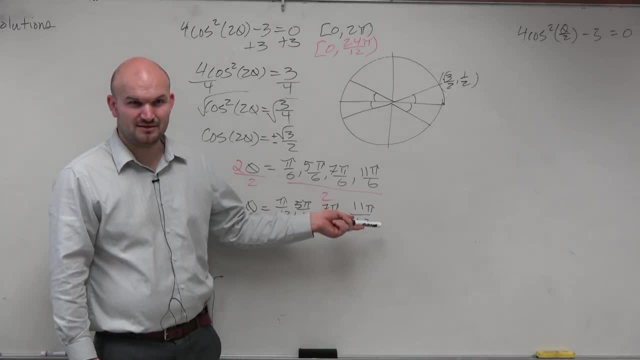 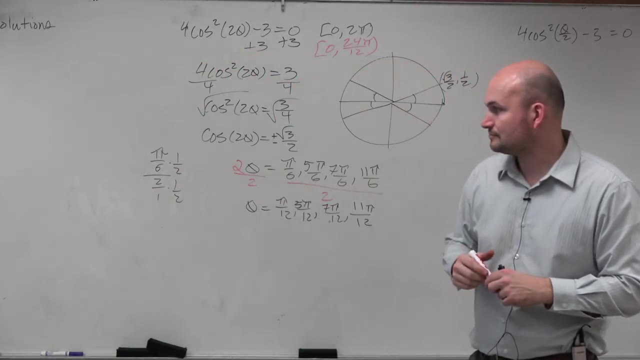 There's room in here for more answers, Don't you guys kind of agree, maybe think So? what I think is helpful to understand this is to understand I'm going to give you an all-solutions answer, which I erased for you, but hopefully you guys wrote down. 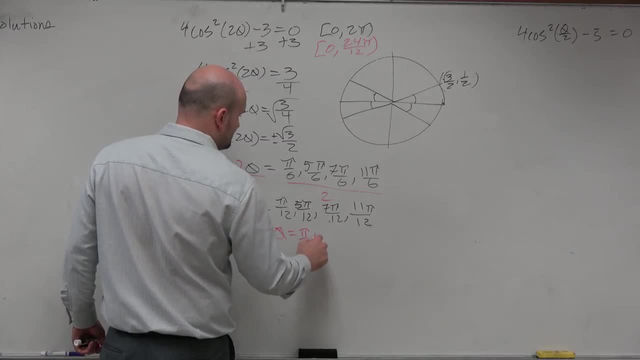 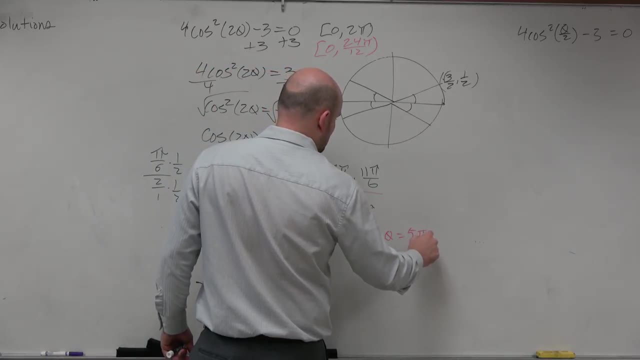 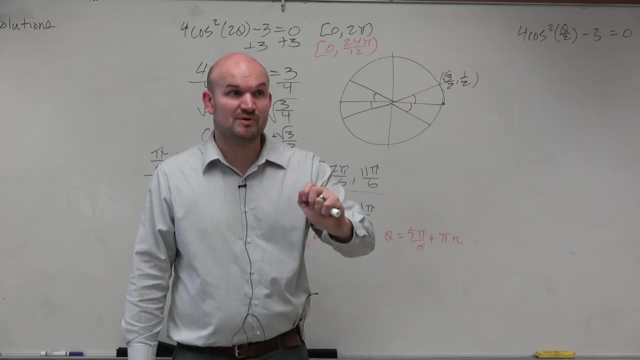 So if I was going to find all the solutions, I said theta equals pi over 6 plus pi n, And then I had theta equaled 5 pi over 6 plus pi n. Remember my simplified answers. Now again, if you didn't do the simplified answers, you would have to do this process to all four of them. 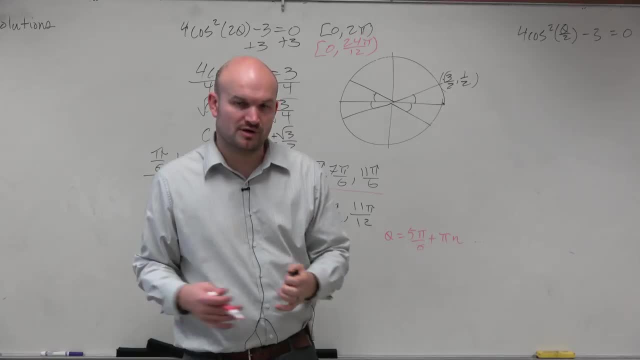 Right, Remember, I showed you guys all four of them and it's like That's what I'm saying: That's way too much work. That's why it's helpful to understand why these simplified answers work. So again, this is from the previous problem. 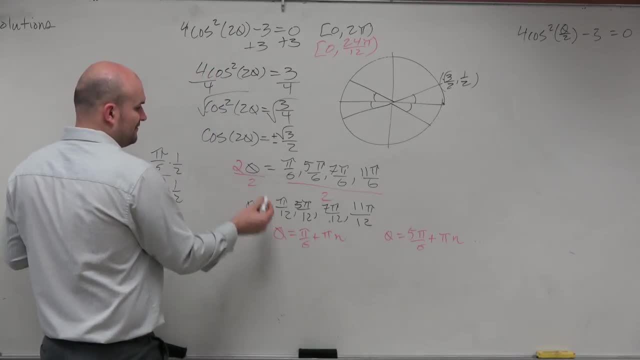 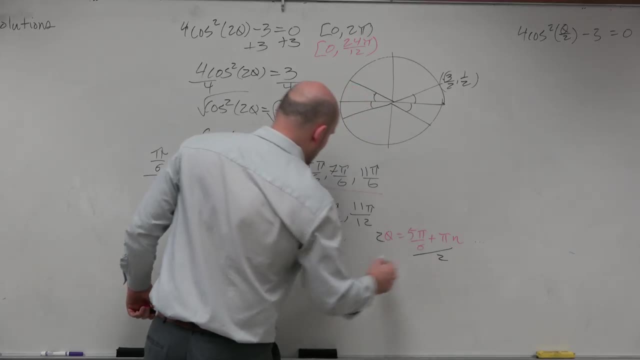 This is representing all the solutions. The difference here is: now we have 2 pi, So you divide by 2 here And again. the more practice you guys get with this, you can actually start doing a lot of this stuff in your head. 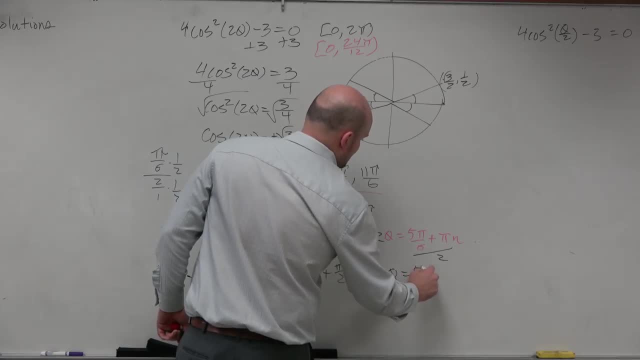 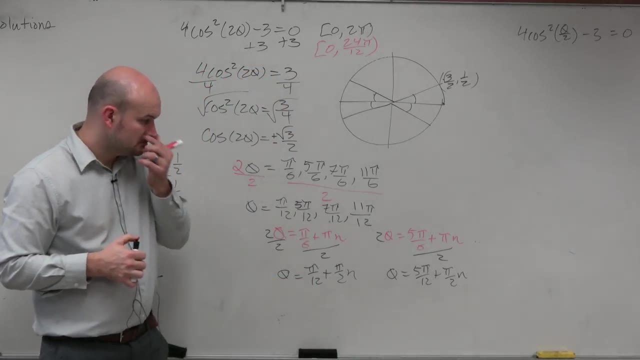 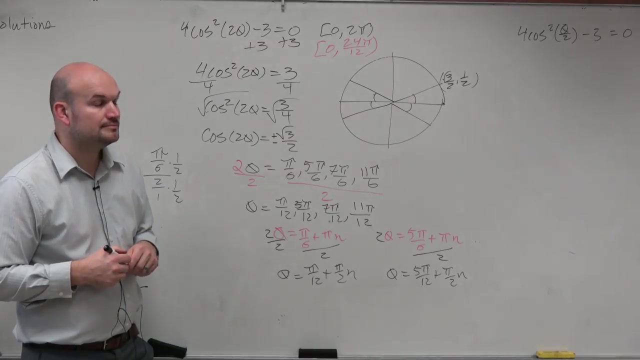 Pi halves n, Pi equals 5 pi over 12 plus pi halves n. Now, Yes, So we're just dividing by 2 here. Say, if it was 3.. It was cosine of 3, theta, Then you do everything but divide by 3?. 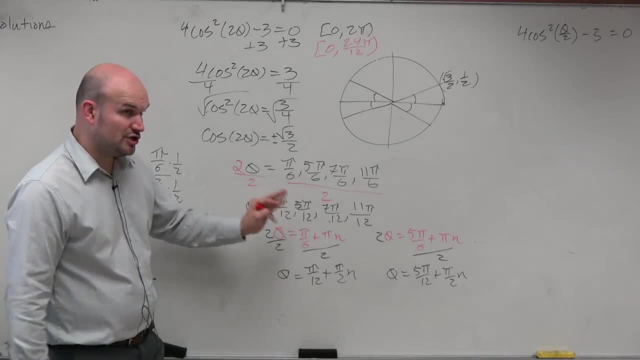 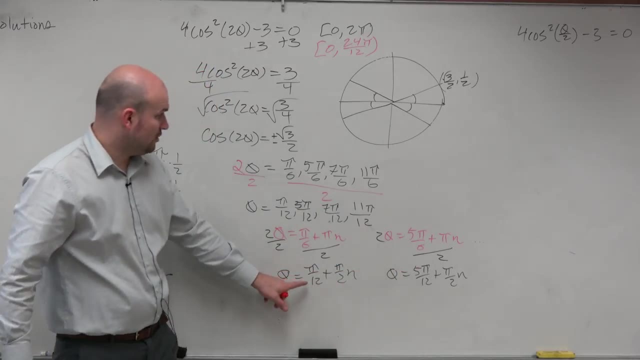 Yeah, But again, remember, we are not done with the answers. And I'm going to show you why we're not done. Again, remember, this represents all the solutions. So let's pretend n is 0.. If n is 0,, what is my answer? 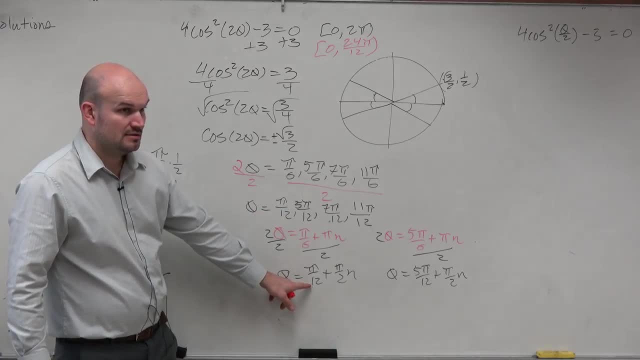 I'm sorry. Divide by 12.. If n is 0,, what is one of my answers? If n is 0,, what's one of my answers? Pi over 12.. Pi over 12.. Do we already have that solution? 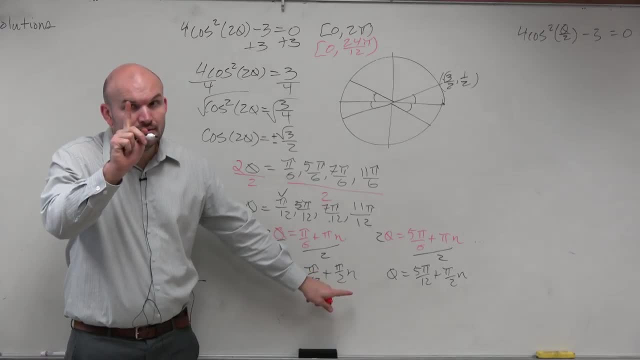 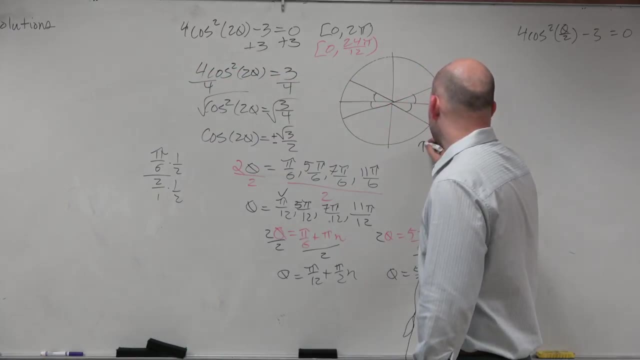 Yeah, So we're good there. What if n was 1?? If n is 1, that's pi twelfths plus 1 half. Now again, it might be helpful to understand: Pi over 2 is equal to 6, pi over 12, right. 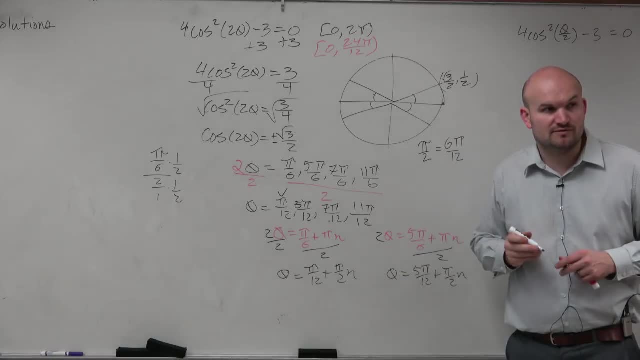 So let's do that. What's 6 pi over 12 plus pi over 12?. 6 pi over 12 plus pi over 12?. 7 pi over 12.. 7 pi over 12.. Do we have that one? 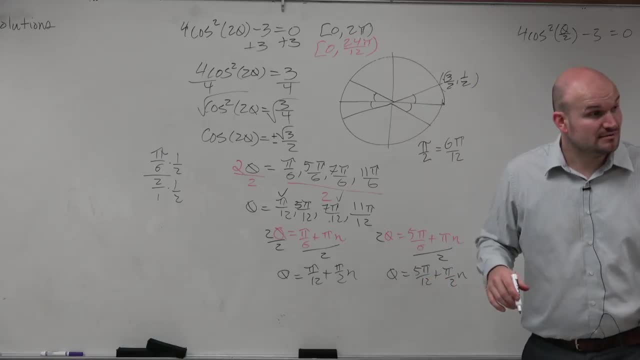 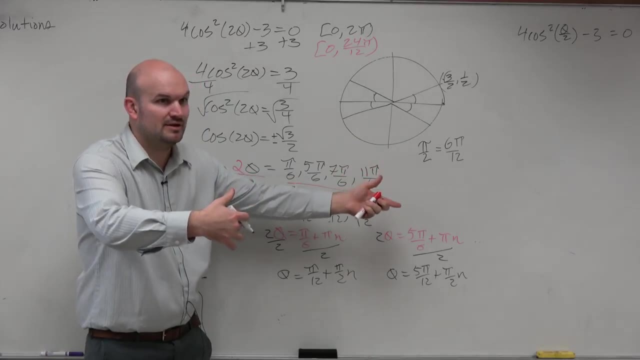 Yeah, OK, Why are you wasting our time? Could we do it again? What if n was 3?? Basically, could we just add 6 pi over that, Like that would be the third time multiplied by 3? Yes, What's 6 pi over 12 plus 7 pi over 12?. 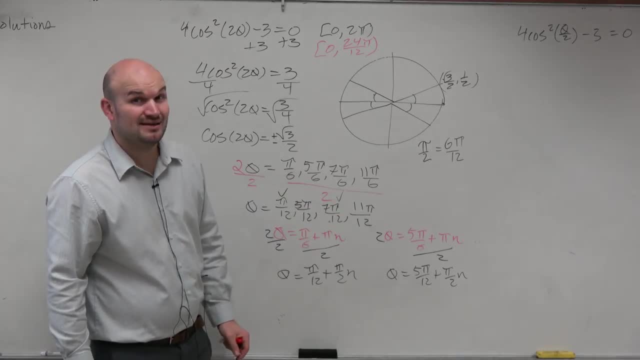 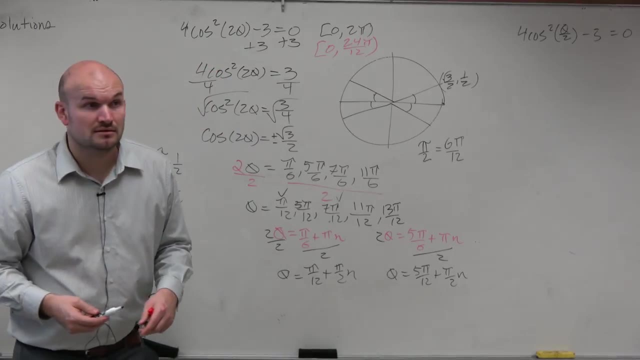 13 pi over 12.. Is that an answer? choice: No, No, But guess what? It is a solution. So you have to add that 13 pi over 12.. Could we do it again? Yeah, We can go all the way up to 24 pi, because that's 2 pi. 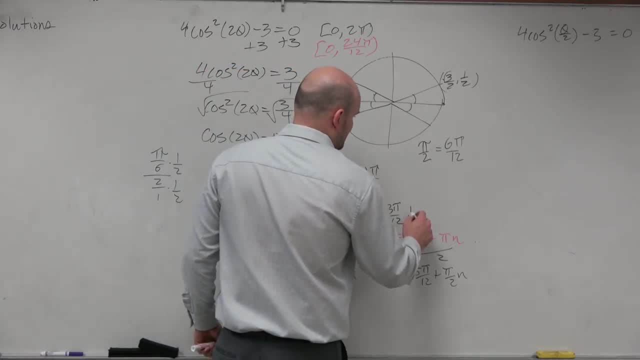 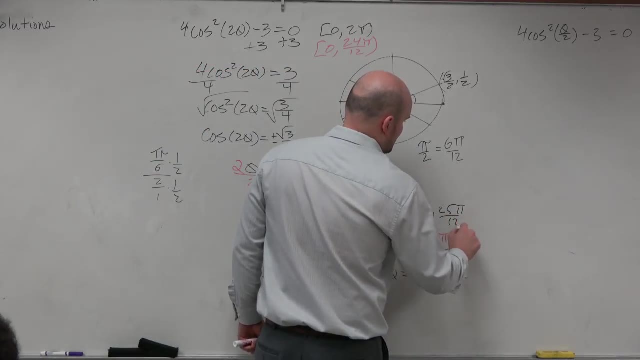 So if we add 6 pi over 12 again, we get 19 pi over 12.. Can we do it again? Yes, Sure. Why not 25 pi over 12.? And then you have to Ah, Ah. 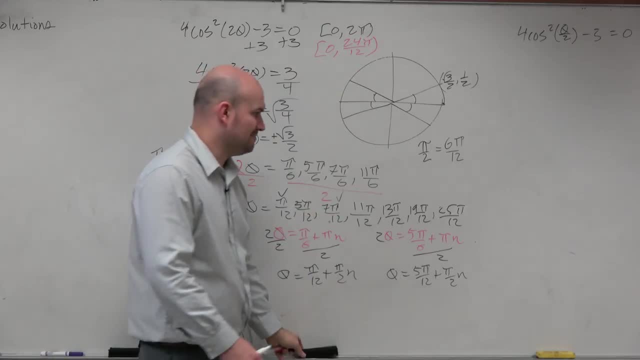 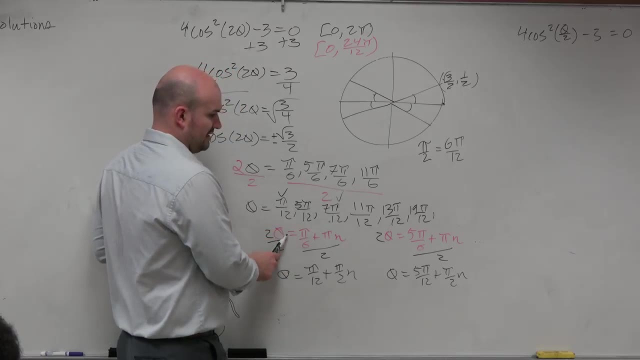 Ah Right, That's above 2 pi, So 25 pi doesn't work. So do you understand how I get where this came from? Do you understand where this comes from? So all I'm doing is n is 1.. 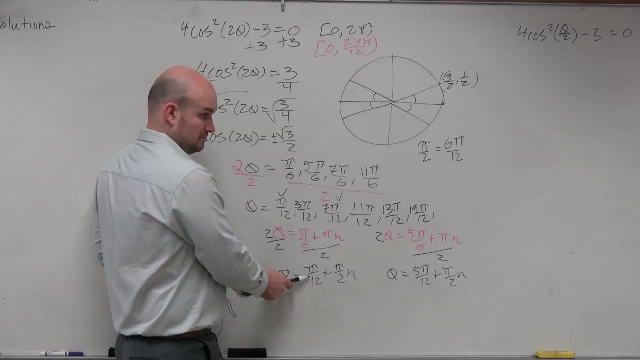 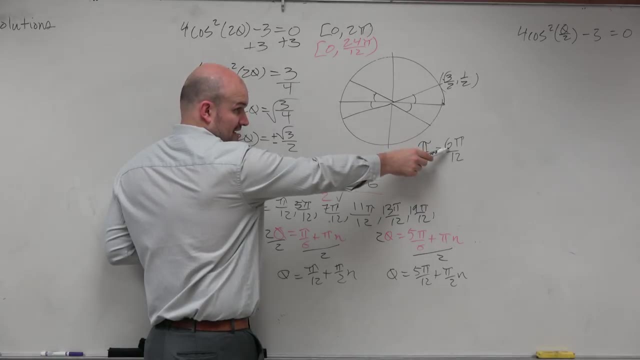 n is 0. You have pi over 12.. n is 1.. 1 times 1 half is 1 half. 1 half is the same thing as 6 pi over 12.. Would you agree with that? So what's pi over 12 plus 6 pi over 12?? 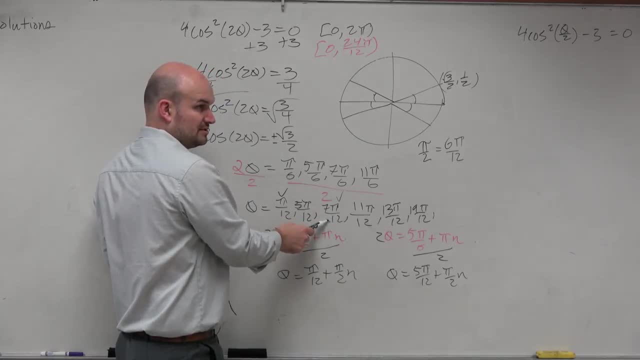 7 pi over 12. You just add the numerators Pi over 12 plus 6 pi over 12 is 7 pi over 12.. Let's add 6 pi over 12 again, because what if n was 3?? 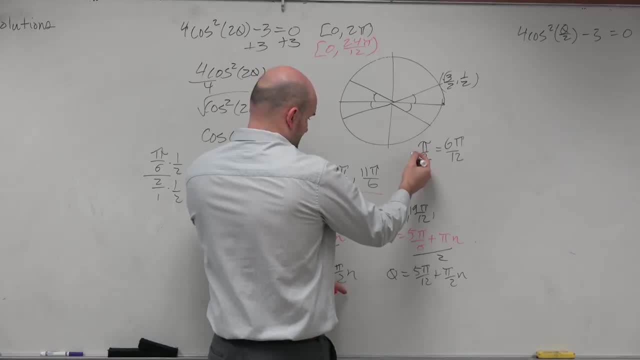 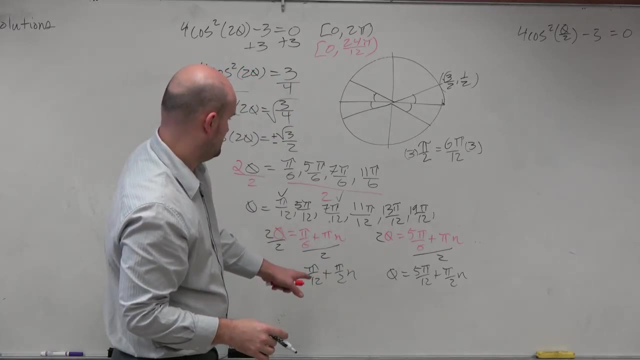 If n was 3,, then it would be. You know, it would be 3 times this or 3 times that, which would be 3 times that, would be 18 pi over 12.. Pi halves Yeah. So if you add 3.. 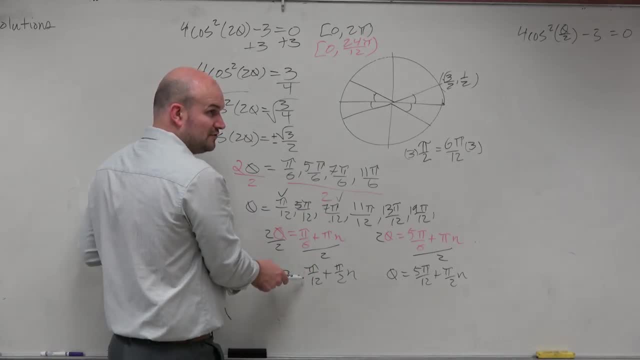 So if you added 18 pi over 12 plus pi over 12,, you would get 19 pi over 12,, which is my answer right there. Okay Now. so we kind of maxed out everything there. Let's do this one. 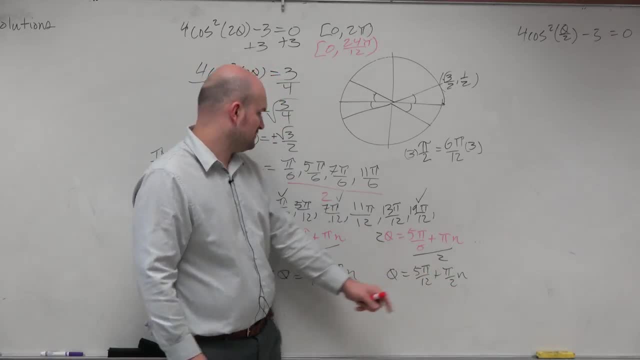 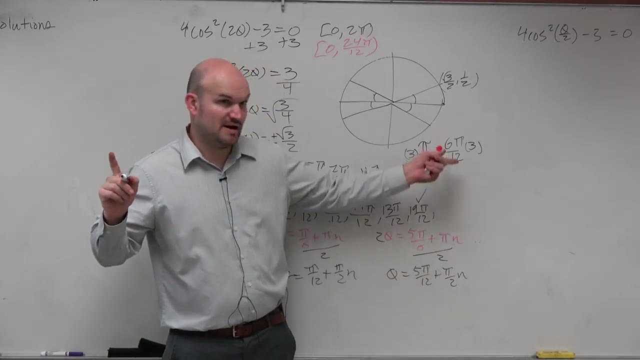 If 5 pi over 12.. If n is 0,, we have 5 pi over 12.. Is that an answer choice? Yeah, We're good. What if n was 1?? So it would be 5 pi over 12 plus 6 pi over 12, which is 11 pi. 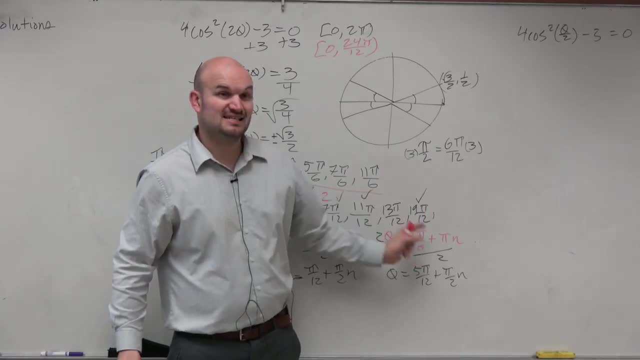 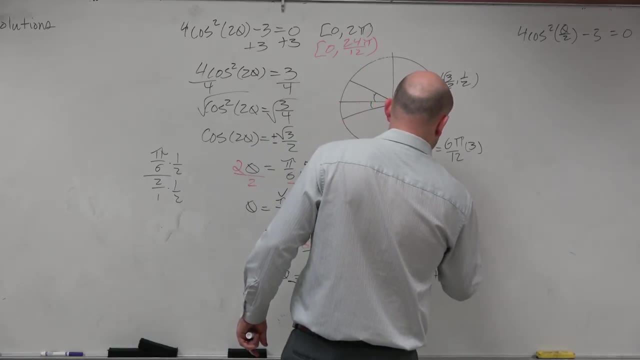 Do we have that? Yeah, We're good. Let's add 6 pi over 12. again, Trying to make it quicker: 17 pi over 12.. Do we have 17 pi over 12?? Nope, That's an answer though.